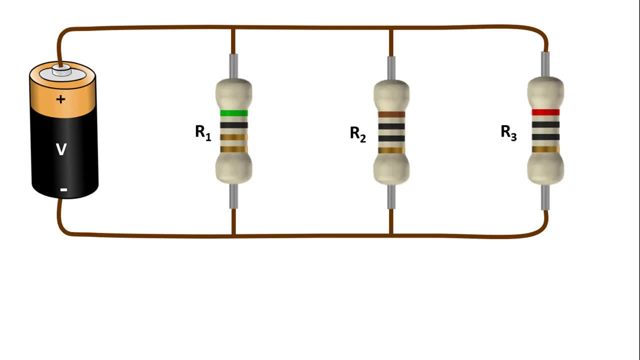 Hi guys, In our previous lesson we examined Kirchhoff's Voltage Law. In this video, I will explain the Kirchhoff's Current Law, which is as important as it is for us to analyze electrical circuits and one of the most important issues we need to know. Let's try to learn this law through. 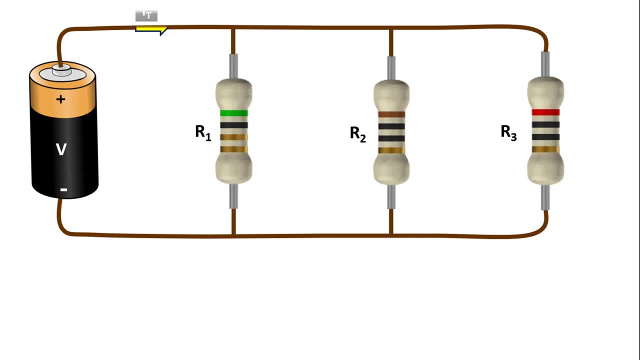 the circuit here. Here let the mains current I t, the current through the R1 resistor Bi1,, the current through the R2 resistor I2, and finally, the current through the R3 resistor I3.. This is where Kirchhoff's Current Law guides us. According to this law, the sum of the currents 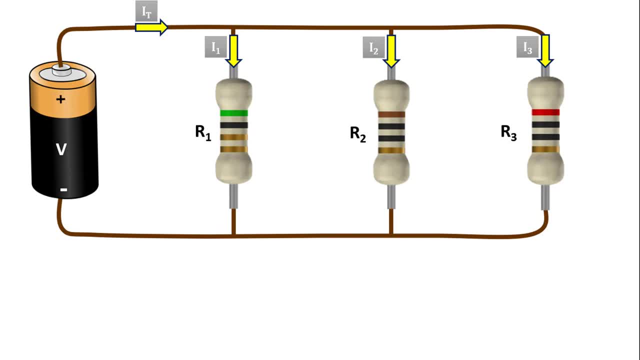 coming to a point is equal to the sum of the outgoing currents. There is only one current coming from the source. here We have shown this current as I t, as the total current, Hence I t will be I1 plus I2 plus I3.. If we assign the value of I t to the right side of the equation, 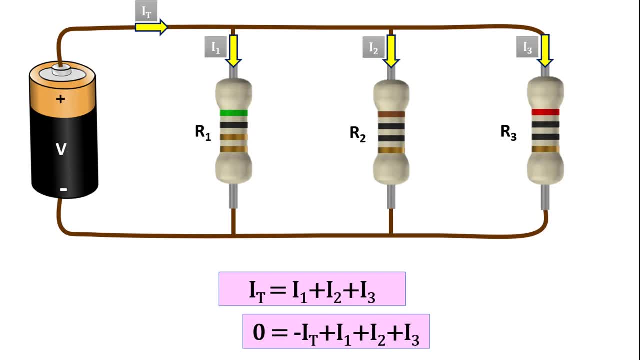 in this formula it will be negative. I t plus I1 plus I2 plus I3 equals zero. So from this formula we can say the following: The sum of all currents in a circuit is equal to zero. Kirchhoff's Current. 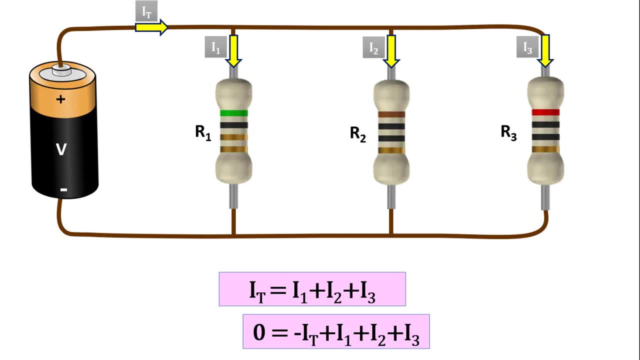 Law is basically like this, friends. Most of the circuit analysis is built on this: The sum of the currents coming into a node is equal to the sum of the outgoing currents, or the sum of all currents in a circuit is equal to zero. Now let's try to understand this formula better through some 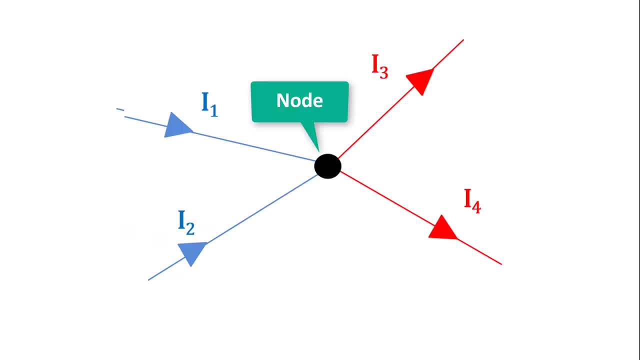 examples. We can better understand what we are saying through the example here. Here are the incoming and outgoing currents to the node. We know that incoming currents are equal to outgoing currents. The incoming currents to this node are I1 and I2, and the outgoing currents are I3 and I4. Then it will be: I1 plus I2 equals I3. 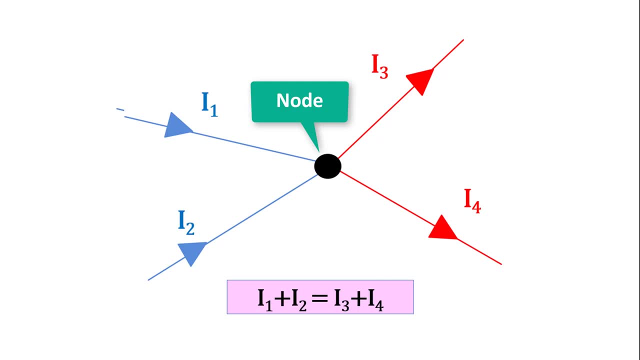 plus I4.. If we add the current values to one side of the equation, it will be zero equals minus I1, minus I2, plus I3 plus I4. That is, the sum of all currents is equal to zero. Thus, while the 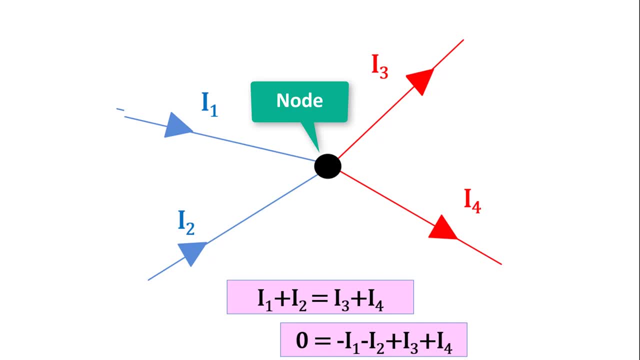 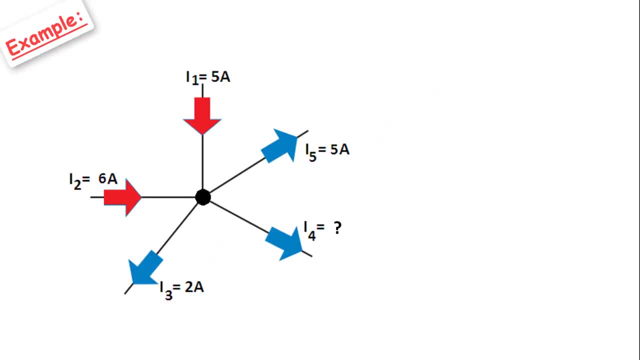 sign of the incoming current is negative, the sum of all currents is equal to zero. If the current is positive, the sign of the outgoing currents is positive. I want you to pay attention to this, guys. What is the unknown current I4 value in this example? 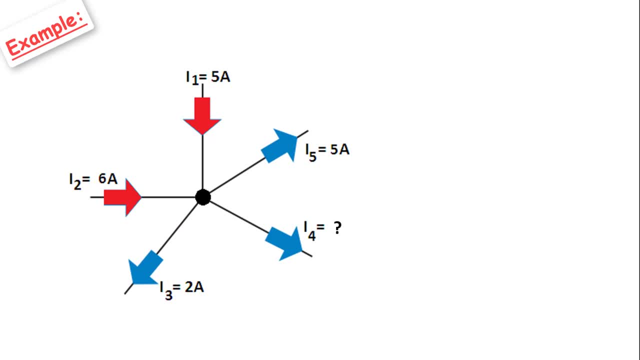 Now let's try to find it. It is seen that the I1 and I2 currents come to the nodal point and the I3,, I4, and I5 currents go from this point. Then it will be I1 plus I2 equals I3. 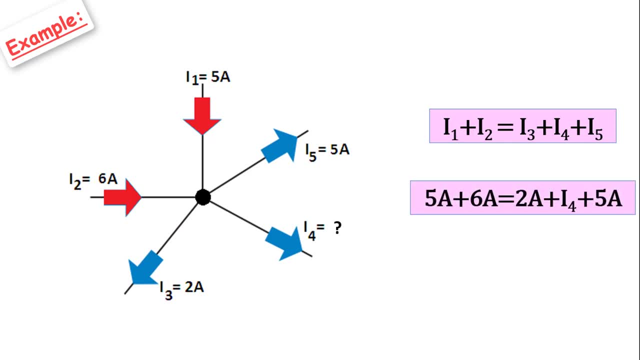 plus I4 plus I5.. If we substitute the values, it will be 5 amps plus 6 amps equals 2 amps plus I4.. From here, the value of I4 will be 4 amps. Now let's do a slightly more difficult example. 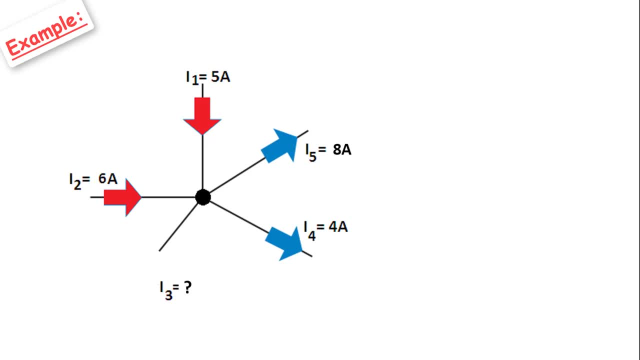 similar to this one, Let this time be an unknown current, I3,, but both its value and its direction should not be known. How do we find the value and direction of this current? We know that, according to Kirchhoff's current law, the sum of the currents flowing into 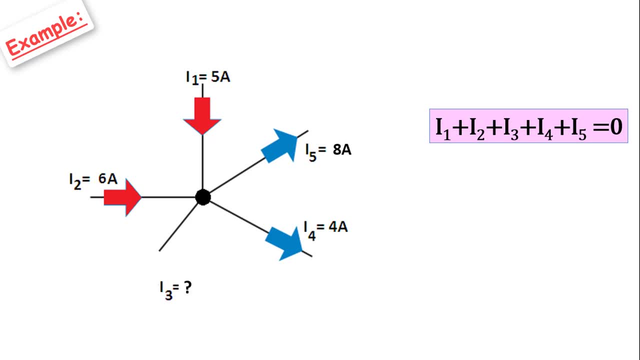 and out of a node is equal to zero. Then we can write the equation: I1 plus I2 plus I3 plus I4 plus I5 equals zero. If we write the incoming currents as negative and the outgoing currents as positive, we can easily find the value and direction of the unknown current. 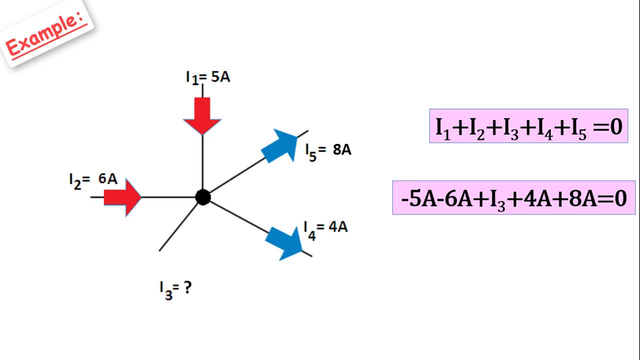 It will be minus five amps, minus six amps, plus I3, plus four amps, plus eight amps equals zero. From here we find the current I3 as negative one amp. So what does the negative mean here? It means that the current I3 is also coming to the node. Its value is 1 k. So when we solve this, we can've find out that 1 is 1 k and therefore the current I3 is now also going to be 1 to the node where its current i3 x per amp to i5 equals. 0 here. So what do we find here? Well, first of all, the minimum value of the current, current I3 values directly belong to the NB, which is a supreme value. Then the number ofV in the part file is usually zero. 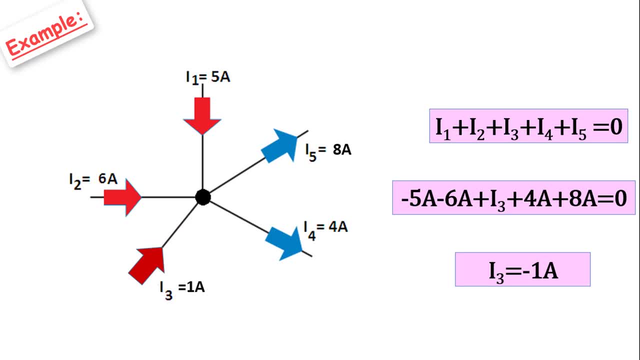 amp. If we found the result positive, we could say that this current is going through the node. Now we can easily see that the incoming currents are equal to the sum of the outgoing currents. Now let's try to find the main sequence current, that is, the total current in this example. 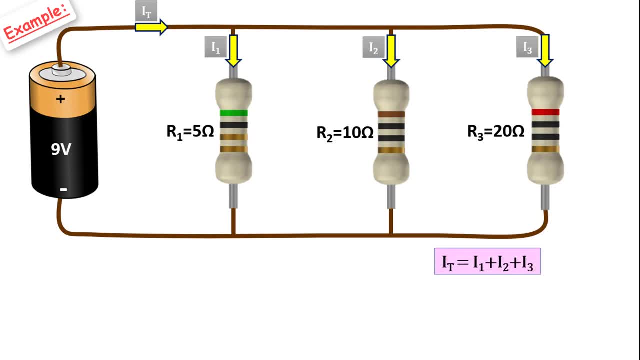 According to Kirchhoff's current law, we know that IT equals I1 plus I2 plus I3.. Then if we find the current flowing through each resistor, we can find the mains current from their sum, Since the resistors are in parallel here.